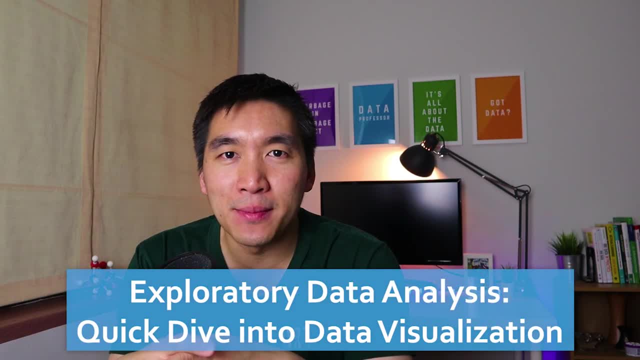 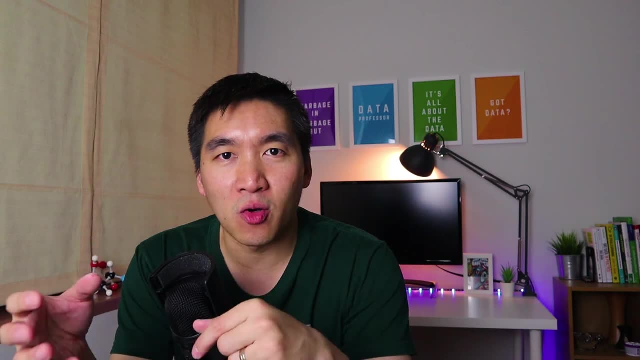 Welcome back to the Data Professor YouTube channel. My name is Chanin Nantat Senamat and I'm an associate professor of bioinformatics And if you're new here on this channel we cover about data science concepts and practical tutorials. So if you're into this kind of content, 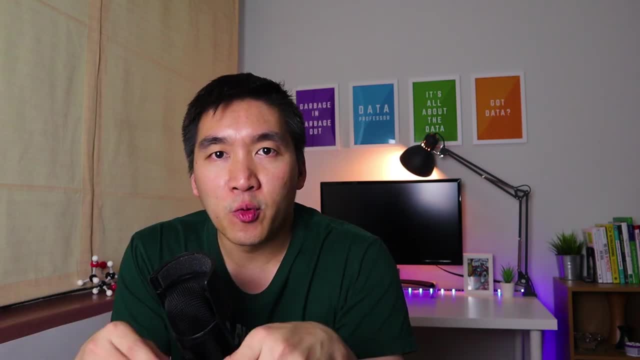 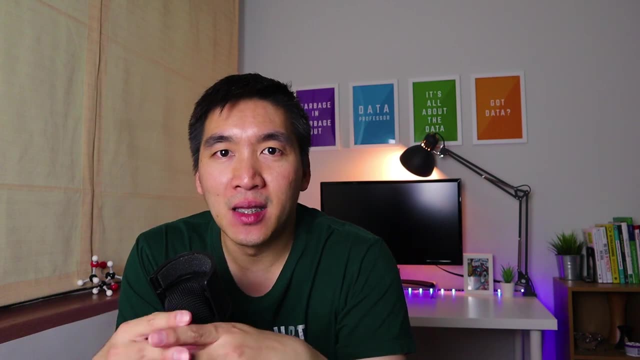 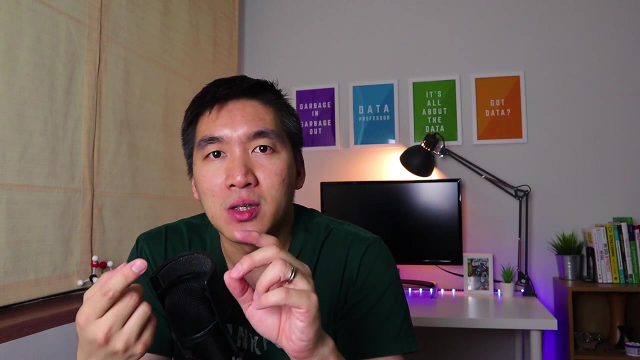 please consider subscribing. In the previous video we have performed exploratory data analysis in order to gain understanding of the data set. So we primarily use the summary function and also the skim R package in order to provide a glimpse of the overview of the data set. 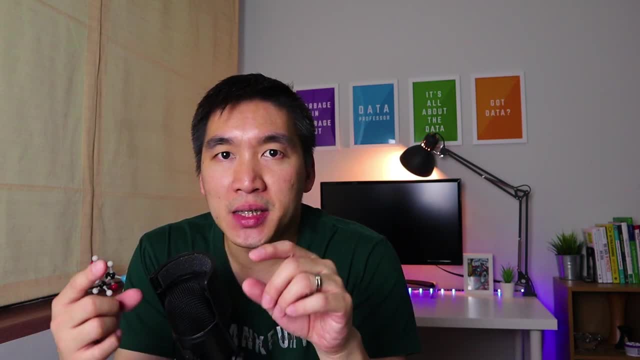 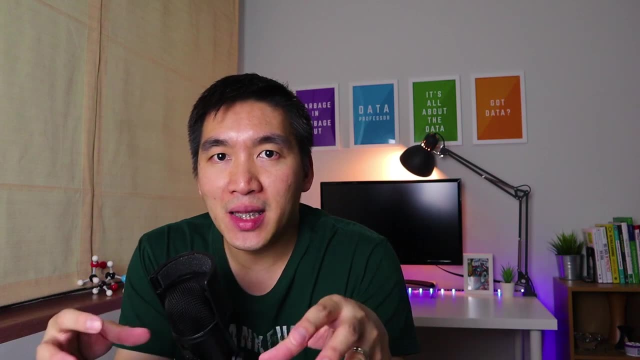 So today we're going to cover additional topics, such as looking more into exploratory data analysis by using the plot function in order to graphically and visually have a look at the distribution of the data itself. So, without further ado, let's get started. 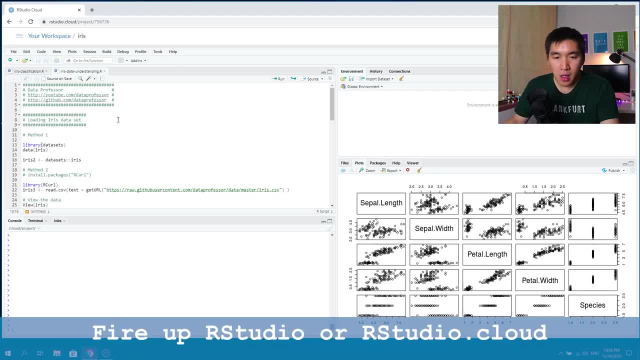 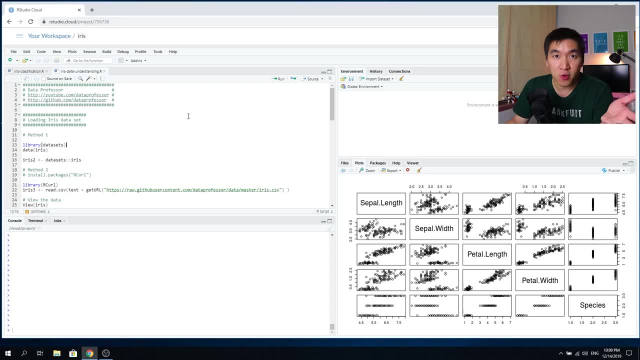 Okay, so fire up your RStudio, whether it be the RStudio dot cloud or the RStudio desktop version, and load the iris data understanding dot r, which is available on the GitHub of the Data Professor. So links down below. on a Windows or a Linux, you will want to hit on the control enter on. 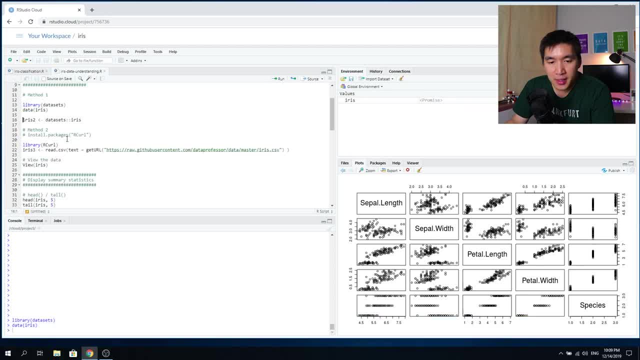 the library data set and then load in the iris data set. As I've told you in the previous video, you have many methods of loading. in this example, data set either method one or method two. Okay, now the data is loaded, So let's scroll to the quick data visualization And we're going to 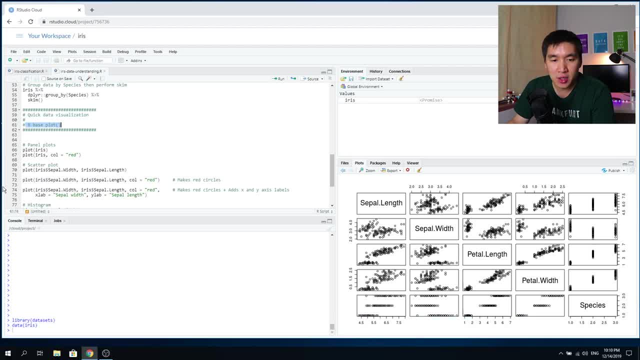 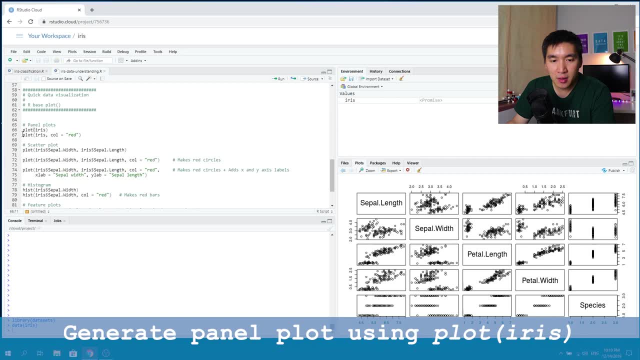 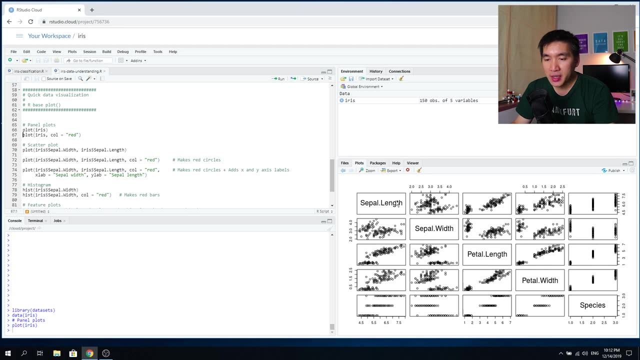 visualize the data using the R base plot function. Okay, so let's enter plot parentheses: iris, so you can easily hit the Ctrl Enter. Okay, and what you will get is this: five by five scatterplot in a pairwise manner between various combinations: 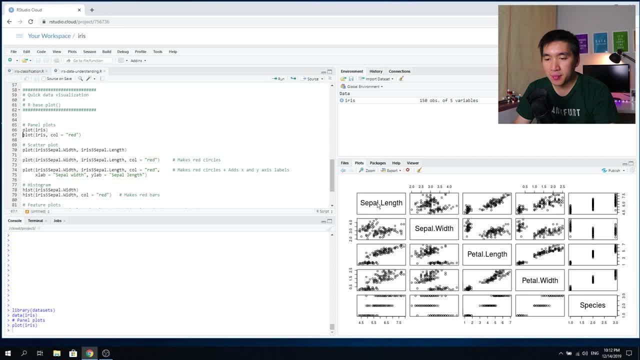 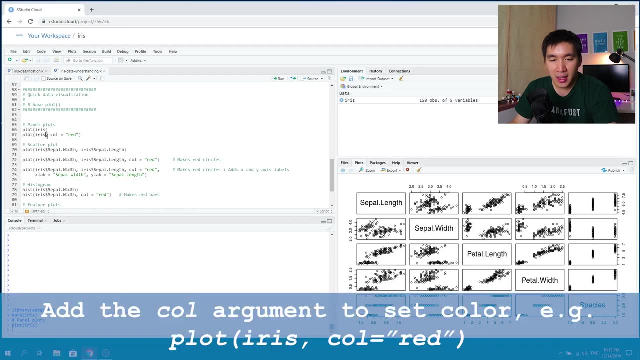 Of the five variables comprising of the simple length, simple width, pedal length, pedal width and the species. Okay, and as you see here, this is the black and white version And if you add another additional argument, adding comma and then col, which is color, equals to red. 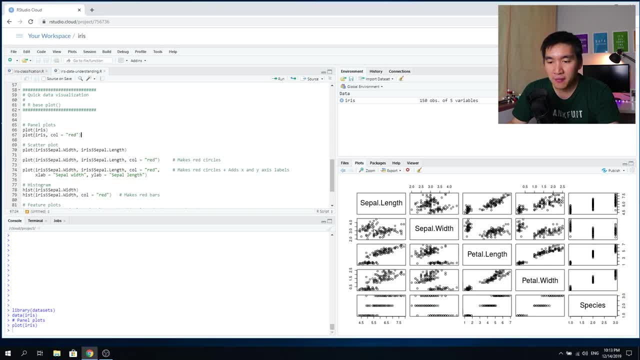 in the quotation mark, you will be able to change the color of the dots to red. So let's give this command a run, And then you see that the dot samples are turned to red color. you can even change it to blue color if you like. So col equals to blue, Ctrl Enter, and then you see it becomes blue color, And so. 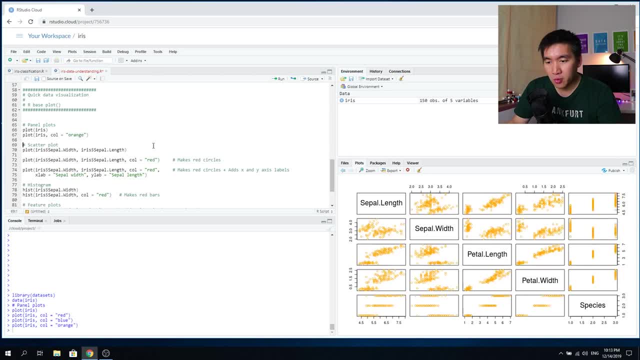 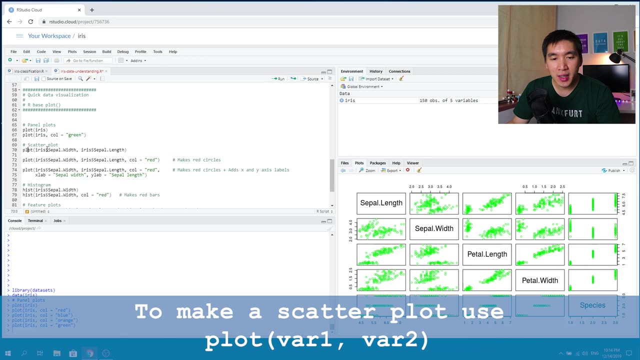 you could change to other color according to your own preference or range, or even green. Okay, if you want to select particular variables that you would like to see in the scatterplot, you can specify it as an argument inside the plot function, So you could. 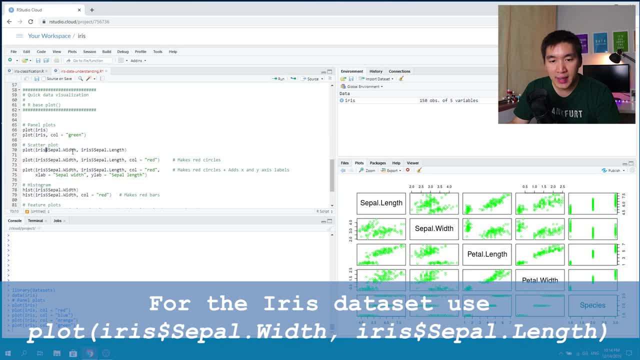 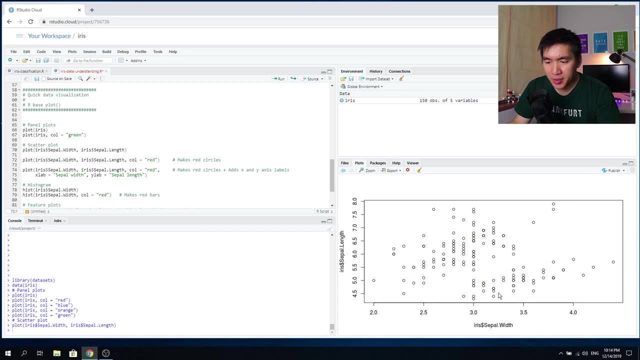 type in iris, and then followed by the dollar sign, and then the name of the variables that you would like to select, which is the sepal dot width, And then you want to have comma: iris sepal dot length. Okay, so you want to Ctrl Enter And then you will see that. 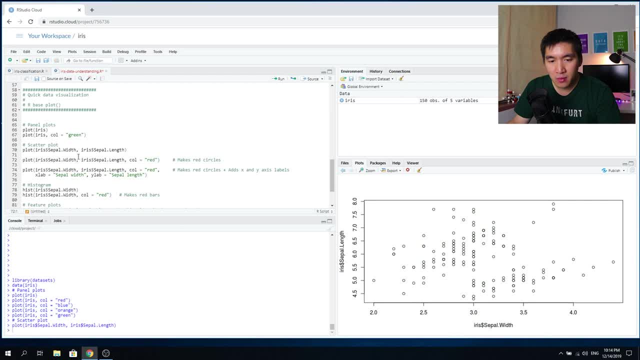 on the x axis is the sepal width, which is the first argument, And then the second is the sepal length, which is the y axis. okay, and you can also add the color argument. gol equals to red and it becomes red. And let's say that you want to add x and y axis labels, although the label will. 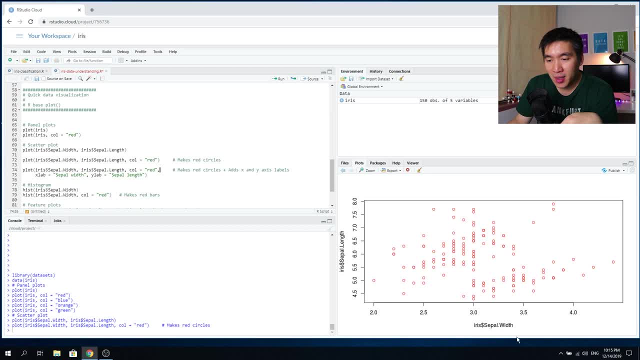 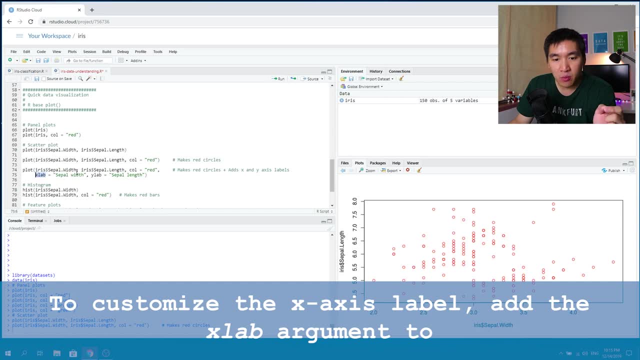 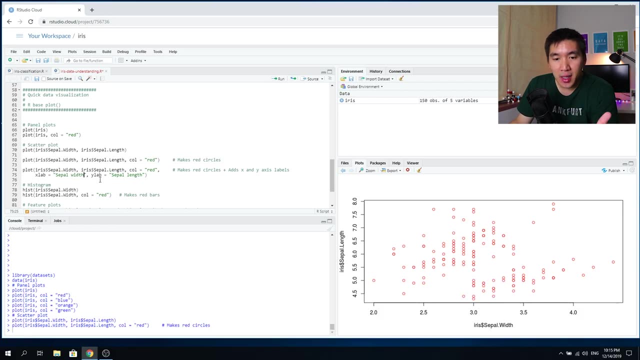 have a default shown here as iris, dollar signs, people with. but you want to customize the label, so you will specify the argument called x lab, equal to the name that you would like to specify in the x axis label. So you could type in, for example, simple width. And in the y lab, which is the y label, you can type in simple link. 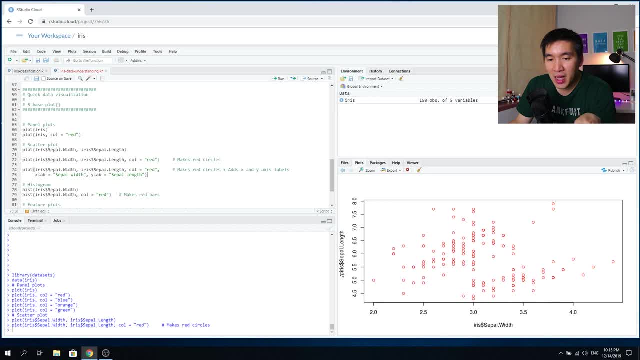 So notice that you don't have the default name, which is Iris dollar sign, simple dot link. okay, which might seem a bit awkward. Okay, so let's run this line of code Control, Enter And you see that the label is already updated so that the simple width is now the x axis label And simple link is. 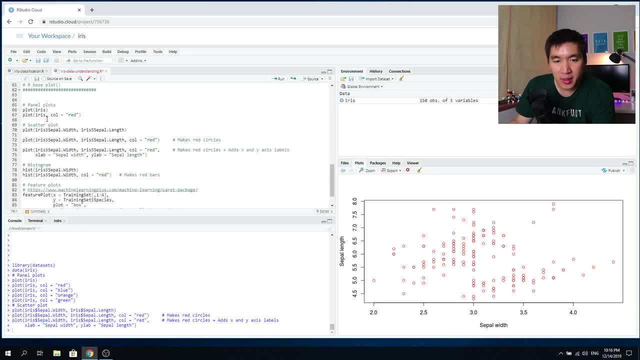 now the y axis label. So what you have seen so far is the, the scatter plot and also the panel plots. the panel plot is the five by five scatter plot of all of the variables in your data set. And now let's have a look at the histogram. Okay, let's say that I want to have a look at the histogram. 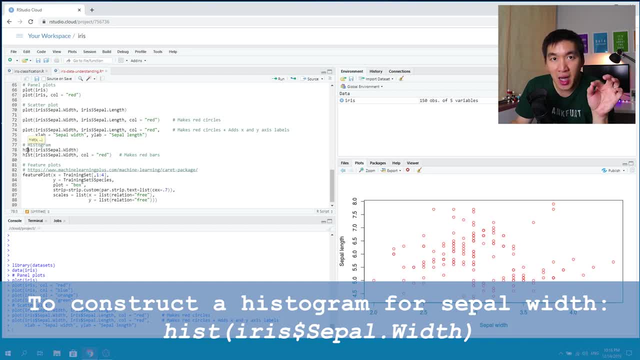 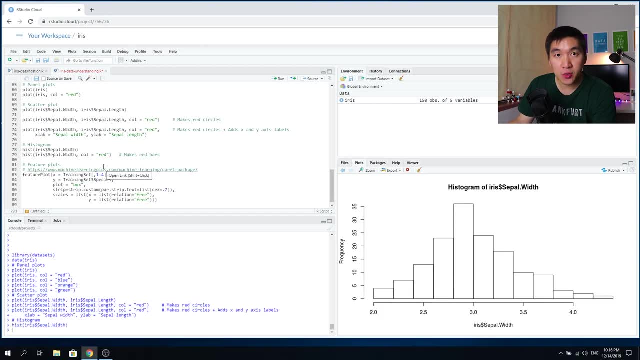 of Iris, simple width. I will type in the function h, i st, parentheses- Iris dollar sign. and then I will type in the function h, i s, t, parentheses- iris dollar sign. And now let's sign simple dot width. So I'm going to enter that in as usual control enter And so notice that. 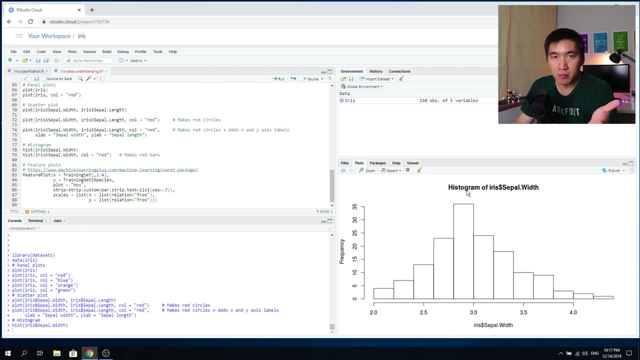 you already have the histogram shown here. What is a histogram, you might wonder? a histogram is a series of bars where each bar represents a range in the value distribution. So the values between 2.0 and somewhere around 2.2 will have a frequency of five. So frequency is essentially the count. 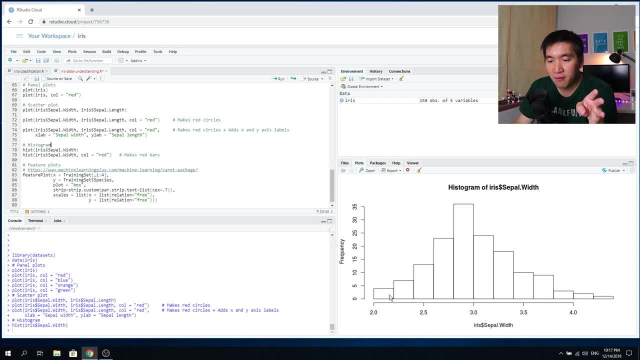 between the range of 2.0 and 2.2, there is a total five sample, and between 2.2 and, let's say, 2.4, there is about seven samples. And between 2.4 and 2.6, there's about 13 samples, And so it is the. 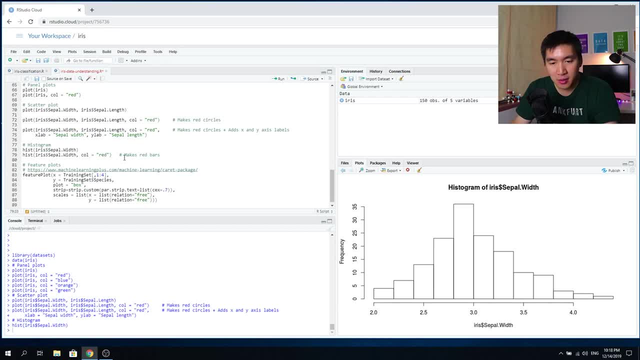 frequency count, And so, as usual, you can add the color red to this histogram, okay, or even make it blue or orange or green. Okay, I'll change it back to red, Okay, so you select a color that you like, And then you can add a color that you like, And then you can add a color that you like. 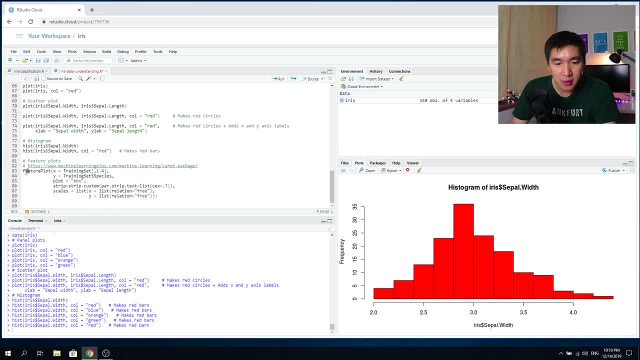 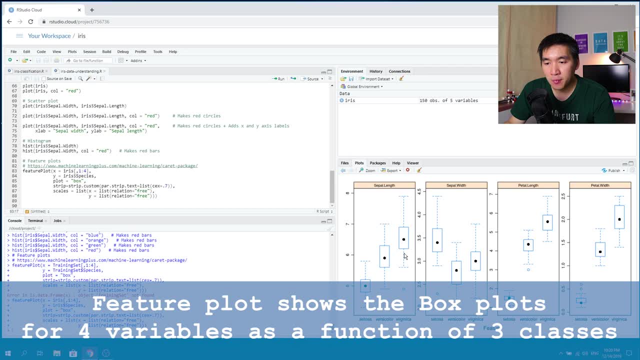 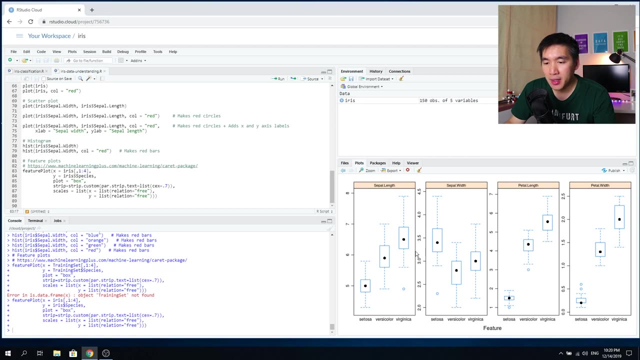 Okay, and let's have a look at the other function called the feature plot. Okay, so the feature plot will allow you to create a box and whisker plot of each of the four variables: simple length, simple width, pedal length, pedal width- And inside is the box plot of. 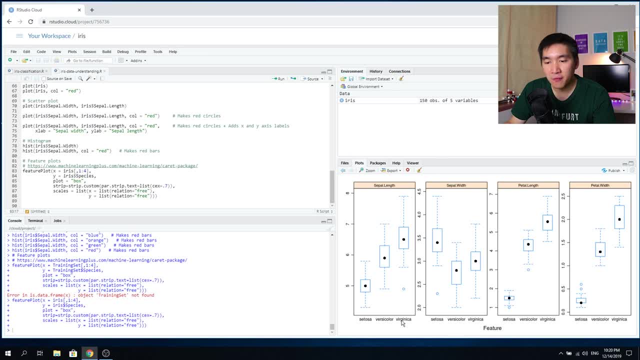 each of the three classes, see Tulsa versus color Virginia. And so for each of the variable we will get to see the relative distribution of the box plot. So we should represents the the q1 and q3 of the data distribution of each of the iris flower class. 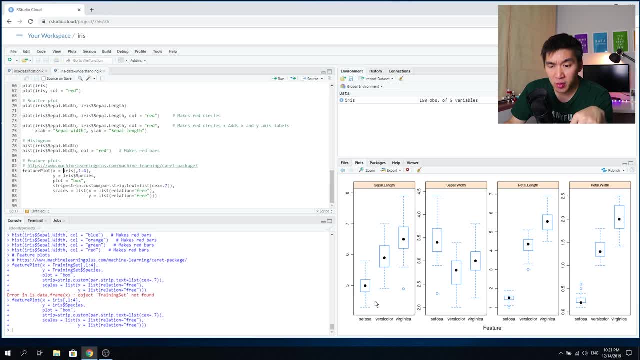 okay, for each of the variable, you will see that for the C Tulsa it has the lowest value amongst the three classes of flower for the simple length descriptor, while C Tulsa has among the highest value for the simple width. and C Tulsa has the amongst the lowest value for the pedal length. 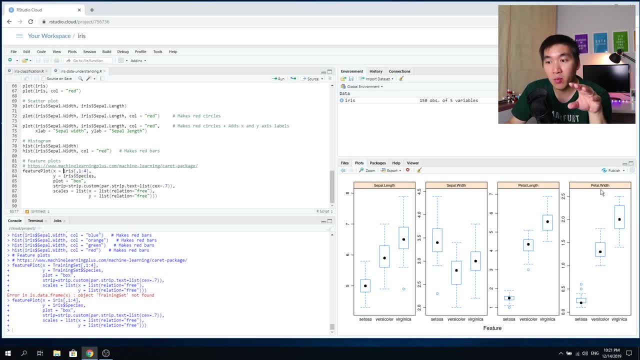 and C Tulsa also has the lowest value for the pedal length and C Tulsa also has the lowest value for the lowest value for the pedal width. and we get to see that for pedal length and pedal width the values of versicolor and virginica are higher than citosa and they're roughly among similar ranges of. 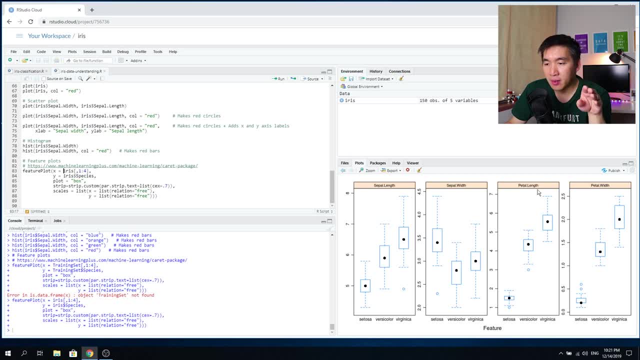 value and the distribution is the same for both pedaling and pedal width with respect to the versicolor and the virginica. okay, and for simple wet, you see that versicolor and virginica have roughly similar distribution, whereas citosa is significantly higher. okay, so you're going to see. 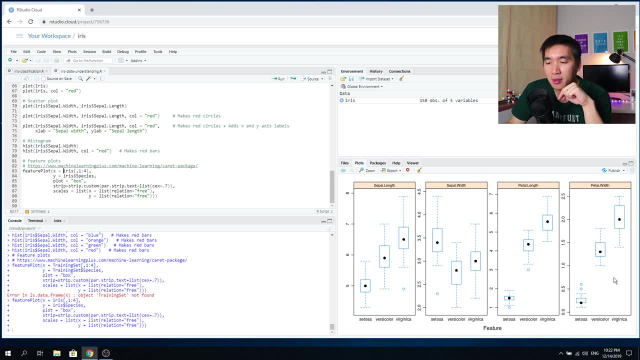 that in all four of the box and whisker plot here citosa is different than the other two flower classes, while the other two flower classes have similar distribution and you will see in the future video, after we have done some model building, you will see that the classes of 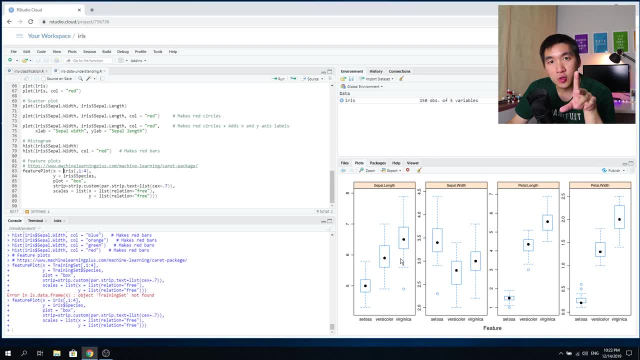 versicolor and virginica. they are mispredicted interchangeably. so for the versicolor and the virginica classes, they are mispredicted interchangeably. so, for example, versicolor might be predicted to be virginica, while virginica is mispredicted to be versicolor, because the underlying features are quite similar for both versicolor and virginica. 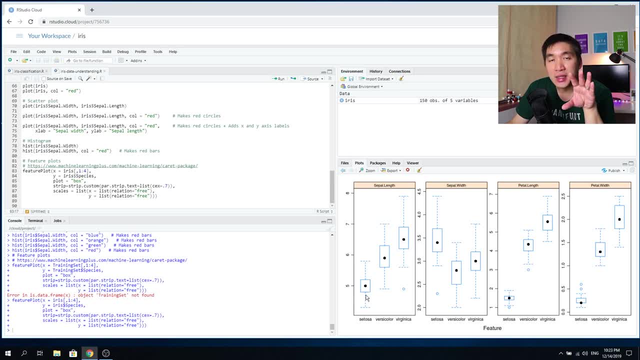 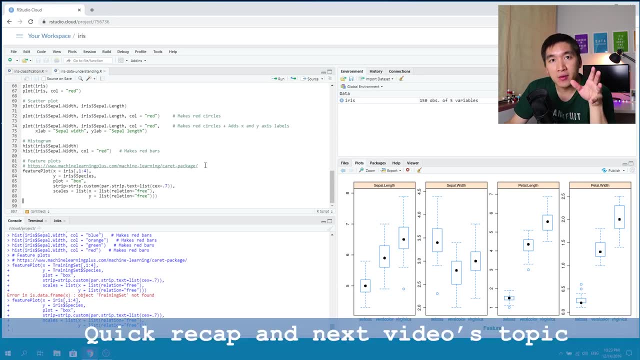 whereas both of them are drastically different than the citosa and therefore the citosa has farther distribution than the two flower classes. so this is it for this video on the data understanding, where we graphically create plots to visualize the distribution of the data, and so in the next video, we're going to cover about how you can build your very own classification. 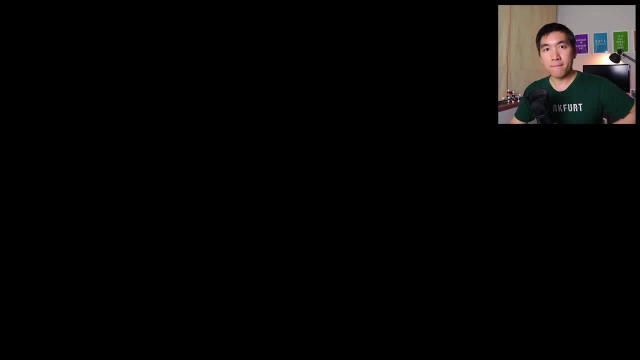 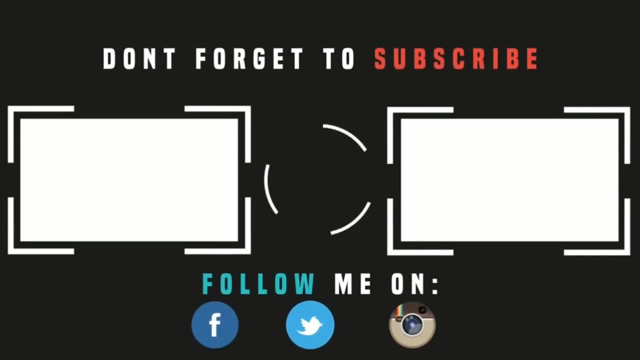 model of this iris data set. so please stay tuned. thank you for watching. please like, subscribe and share and i'll see you in the next one, but in the meantime, please check out these videos.